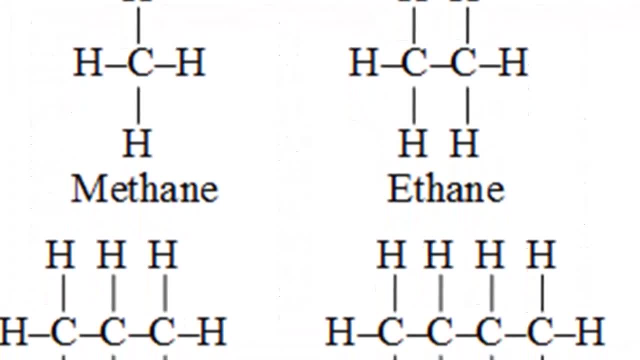 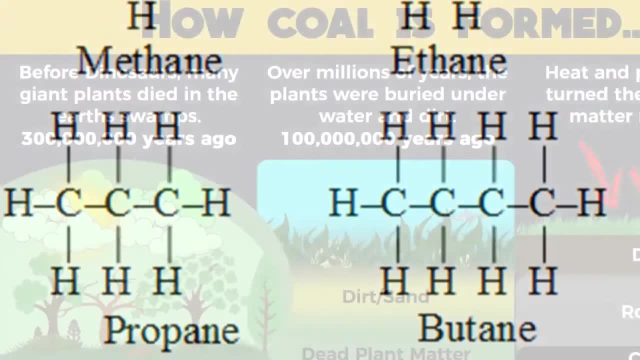 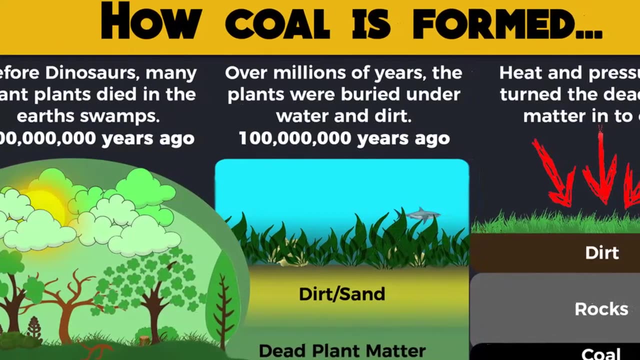 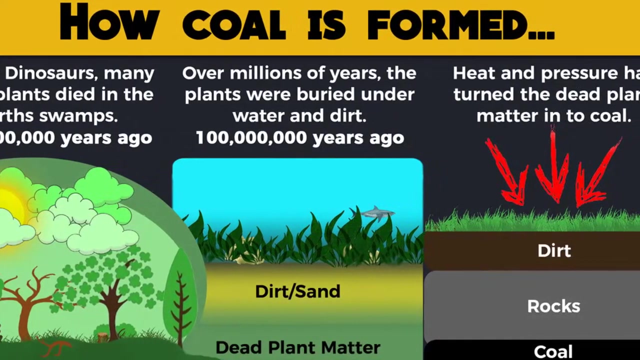 Like coal, petroleum and natural gas are biological products derived from the remains of organisms. However, the environments in which they form are very different, as are the organisms. Coal is formed mostly from plant material that accumulated in a swampy environment above sea level. 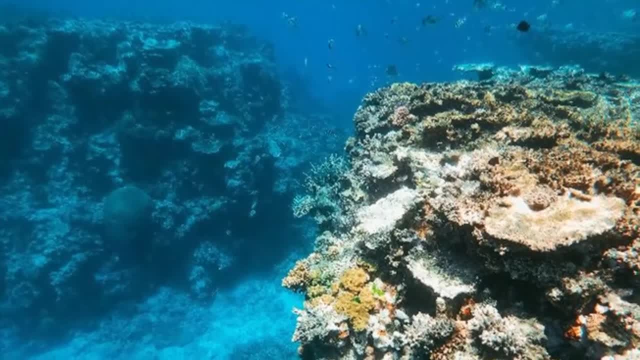 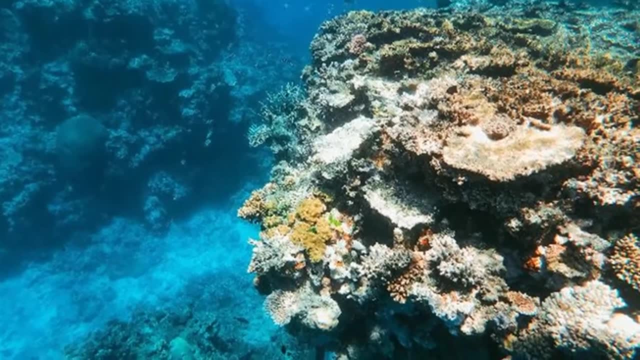 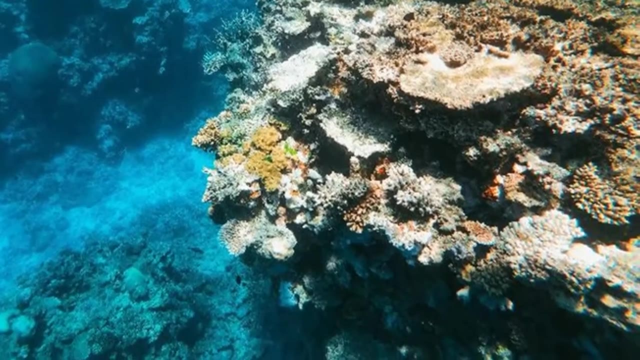 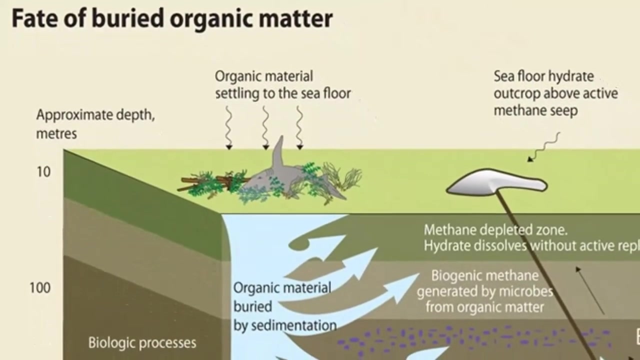 Oil and gas are derived from the remains of both plants and animals having a marine origin. Petroleum formation is complex and not completely understood. Nonetheless, we know that it begins with the accumulation of sediment in ocean areas that are rich in plant and animal remains. 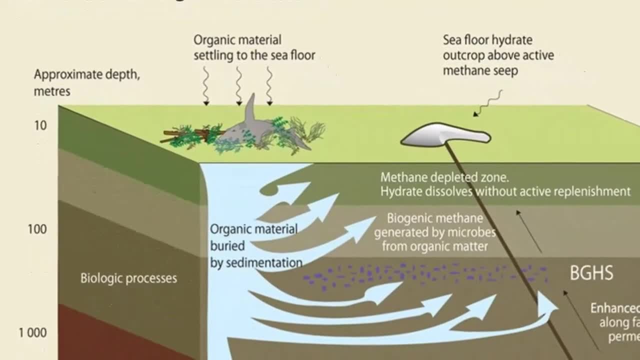 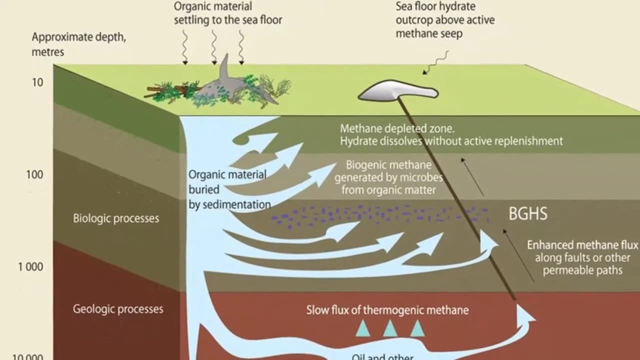 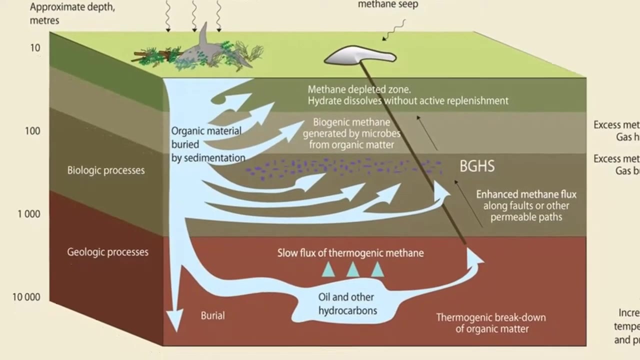 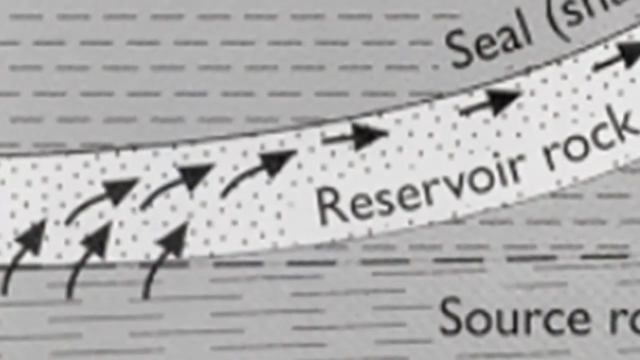 These accumulations must occur where biological activity is high, such as in near-shore areas. Most marine environments are oxygen-rich, which leads to the decay of organic remains before they can be buried by other sediments. Therefore, accumulations of oil and gas are non-existent. 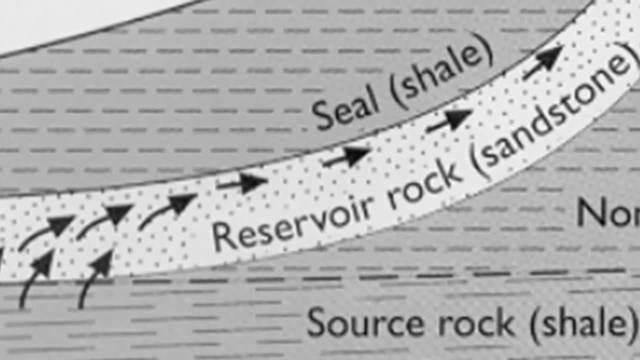 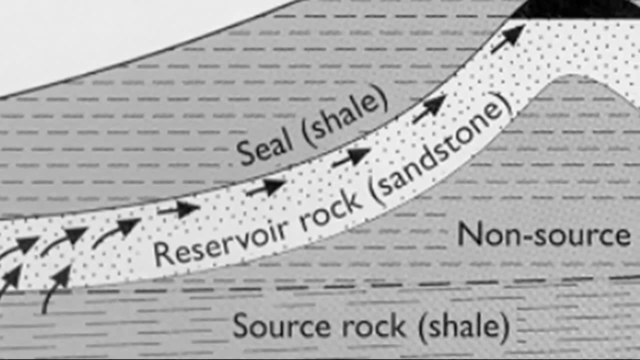 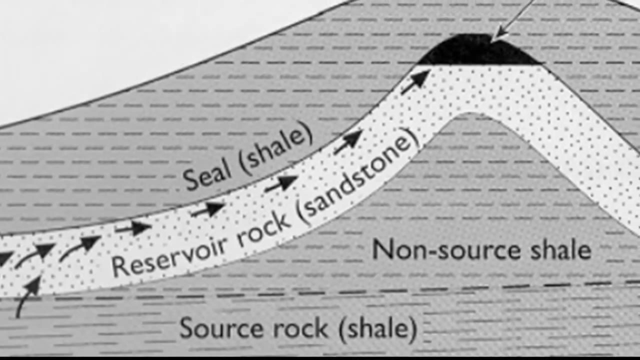 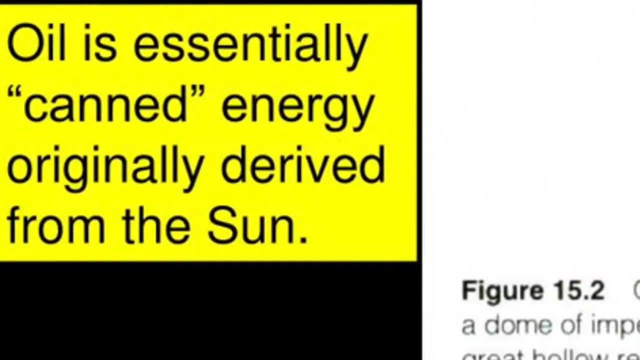 The amounts of oil and gas are not as widespread as are the marine environments that support abundant biological activity. This limiting factor notwithstanding, large quantities of organic matter are buried and protected from oxidation in many offshore sedimentary basins, With increasing burial over millions of years. 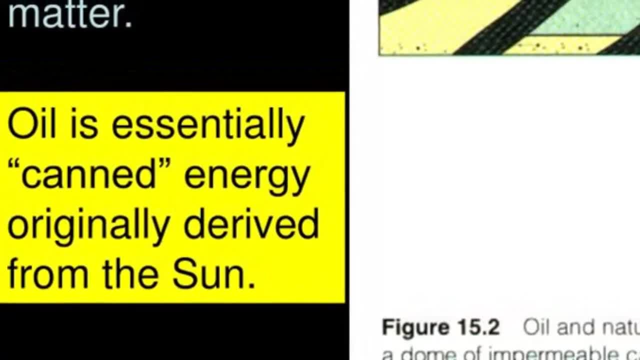 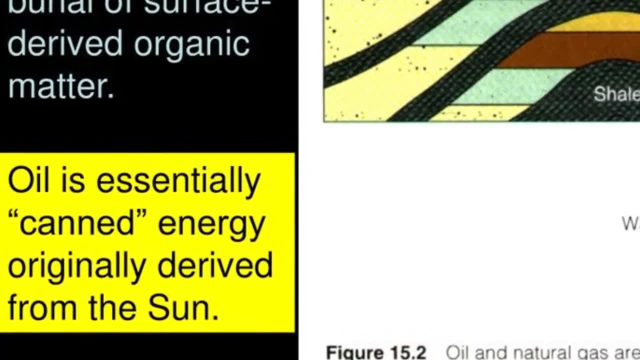 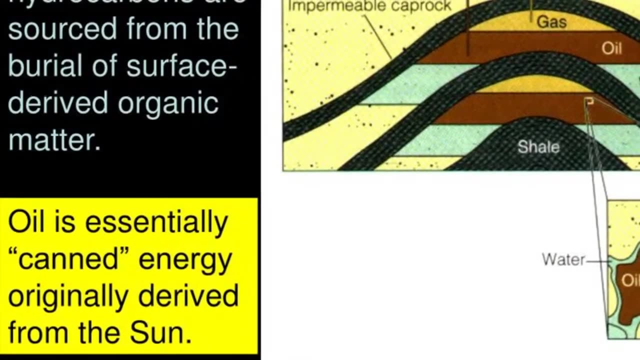 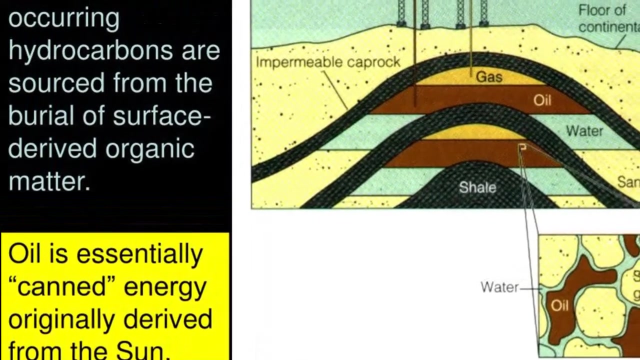 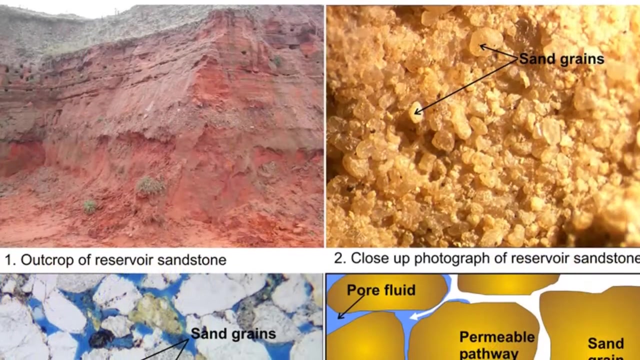 chemical reactions gradually transform some of the original organic matter into the liquid and gaseous hydrocarbons we call petroleum and natural gas. Unlike the organic matter from which they formed, the newly created petroleum and natural gas are mobile. These fluids are gradually squeezed from the compacting mud-rich layers where they originated.